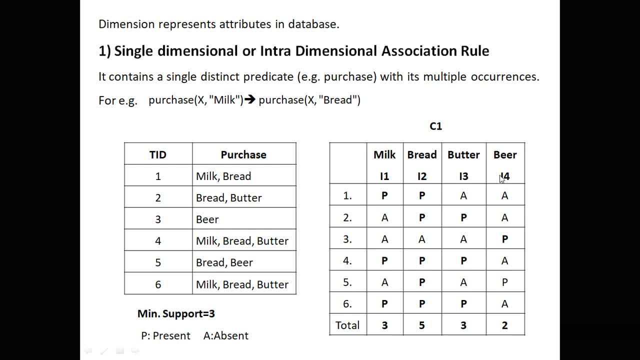 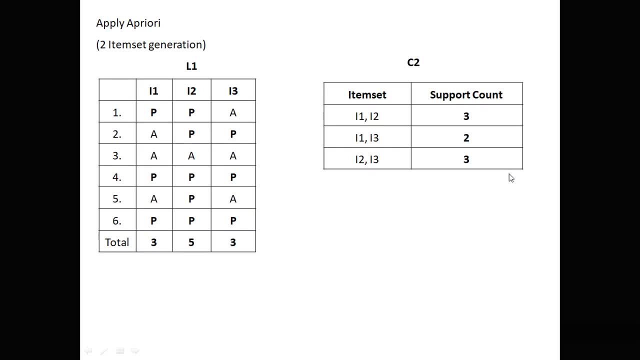 l1 by using a priori algorithm. now here in l1 beer is excluded because it does not satisfy the minimum support count to item set generation. that is a next time. for that our input is l1. now in l1, i4 column gets cut because it does not satisfy that property. 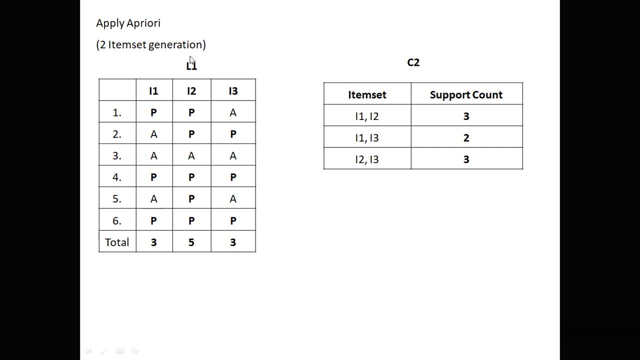 now from l1 we are generating the c2. that is two items at generation. so i1 i2, i1 i3 and i2 i3. now we require to count in the table how many times it comes. so for example, i1 i2 coming for. 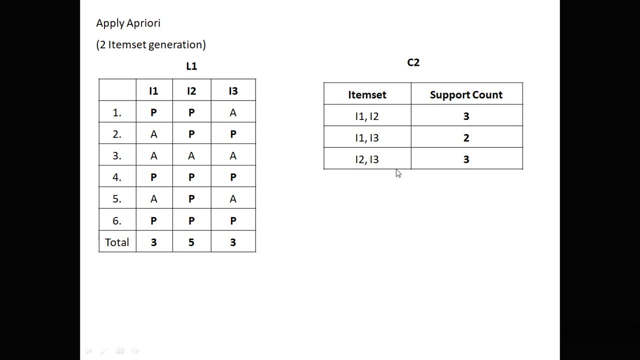 three times: i1, i3 two times and i2, i3 three times. now this is our c2. from c2 we generate the l2. l2 will take all records because all satisfy the minimum support count. this is uh sorry. minimum support count is three. therefore i1 and i2 is excluded from the l2. so in l2 we are getting 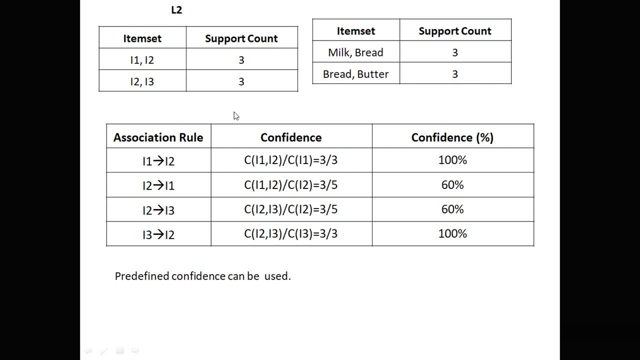 only two combination: i1, i2, i2, i3 with the support count three: i1, i2 is nothing but the milk and bread and i2 is nothing but i2. i3 is bread and butter. so there is support count is three here. three item set combination is not possible. 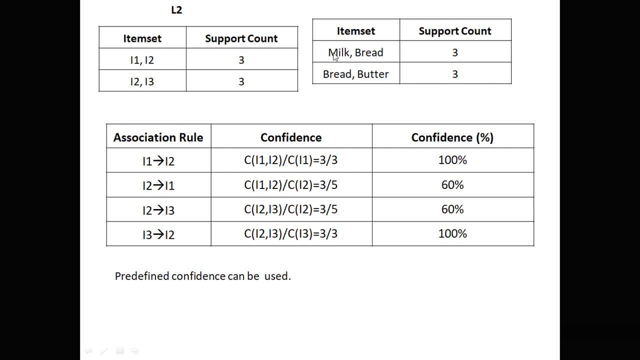 because for to generate the three item set combination we require, first item must be common. Now from this we can generate the rules. For example: i1 implies i2, that is count of i1. i2 divided by count of left side, that is i1, 3 by 3. 100 percent. i2 implies i1: count of i1. i2 divided by count of i2.. So in 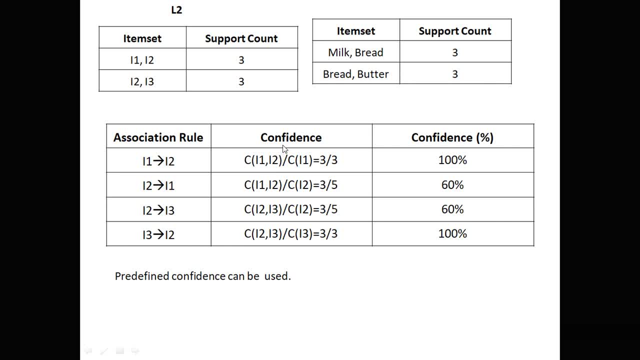 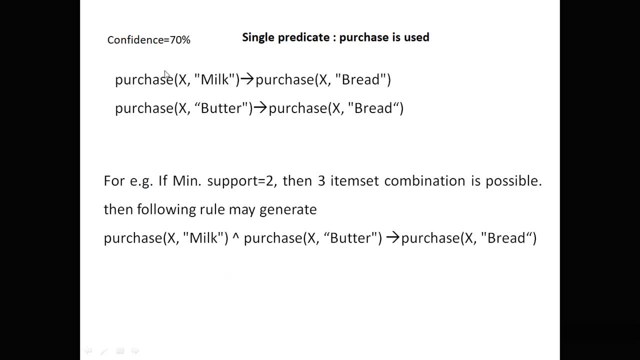 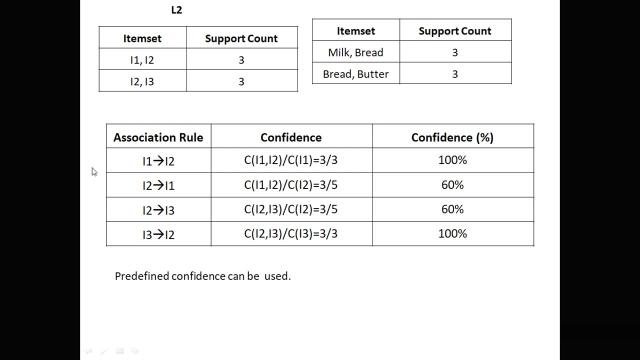 this way we can apply the rules and using the formula of confidence, we are getting the particular confidence. Predefined confidence can be used, for example, here i am using the confidence as 70 percent. Now, if we apply the 70 percent confidence, we are getting only two rules: i1. 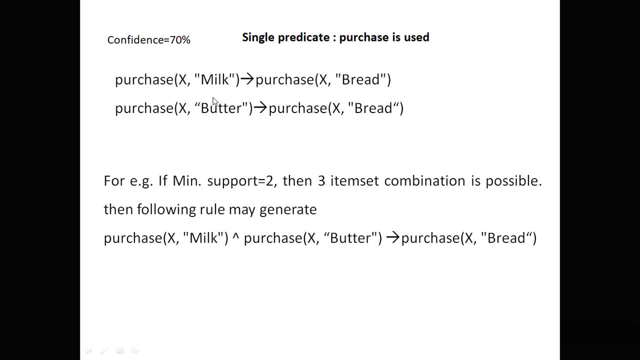 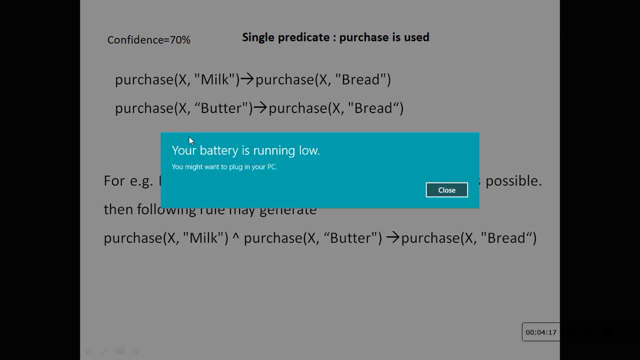 implies i2 and i3 implies i2. that is nothing but milk implies bread and butter implies bread. So in this way we can generate single dimensional, multi, single dimensional association rule where the predicate purchase is repeated. Now for the same example: if minimum support count is 2, then three item set combination is: 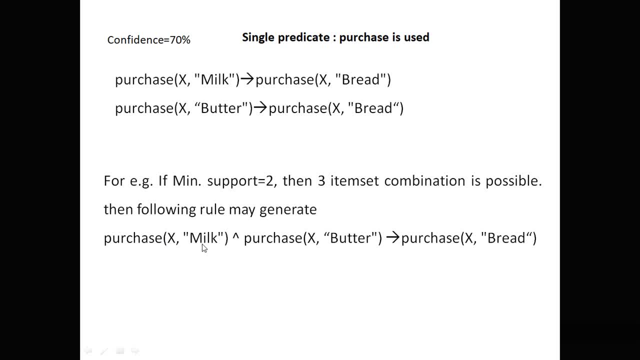 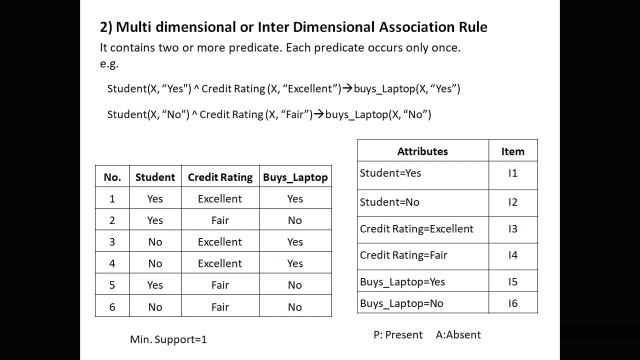 possible. and then the following rule may generate that: milk and butter implies a bread. So you just try for this example with minimum support equal to 2. that can be a very good exercise. Second is multi-dimensional or inter-dimensional association rule. It contains two or more predicate each. 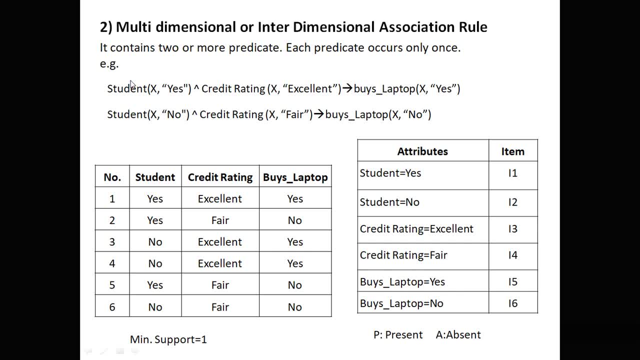 predicate occur only once. For example, predicate here is student and credit rating and vice computer. They occur only once Now: student yes, credit rating excellent, Vice computer yes. Second rule is: student no, credit rating fair and vice-laptop no. Now we will see how to. 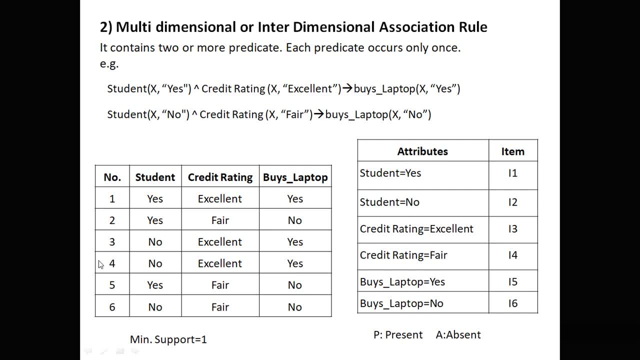 generate such type of multi-dimensional rules. Just take a simple example. Six records are there. Student credit rating are the two attributes and vice-laptop is our final classification. level category is yes or no. so for that we generate the two items. that is student. yes is as i1 student. 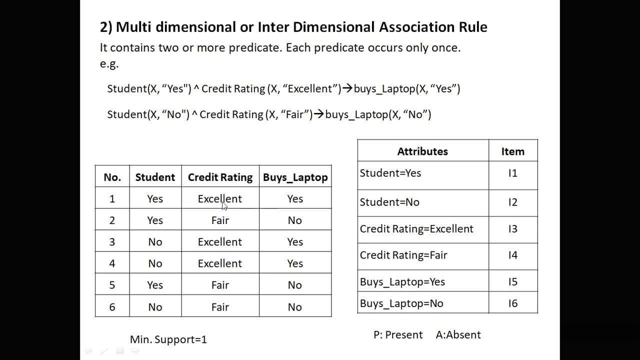 no as i2 credit rating. two categories are there. so credit rating excellent: is i3, credit rating fair: is i4 for buys laptop, yes is i5 and no is i6. so again we are using the convention like p for present and a is for absent, and making the c1 table. here minimum support is equal to one now. 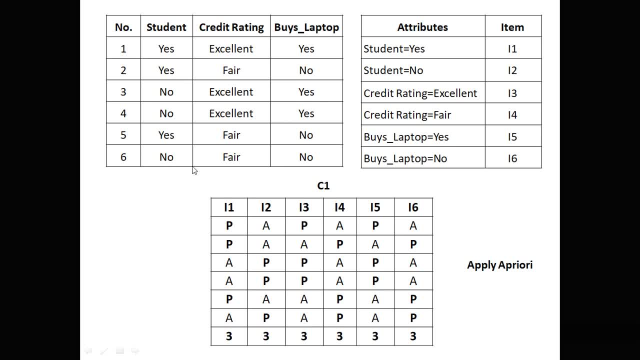 c1 generation. i am explaining you other for the first record. you can easily understand for the rest of the record. first record is yes, excellent, and yes, now s that is, i1 is present. now see when i1 is present. i2 can be absent only because this is yes, no combination. so i2 is a credit rating is 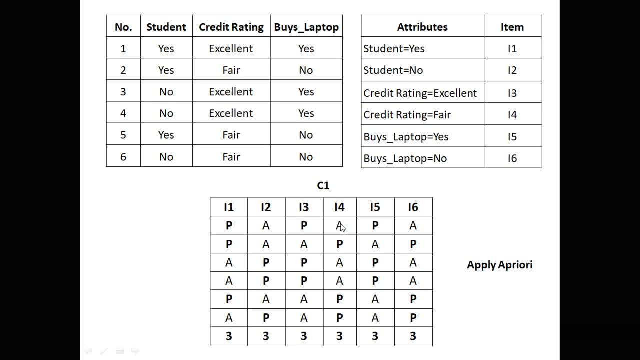 excellent is nothing but i3. so i3 present when i3 is present, compulsory. i4 is absent and i4 is upset and i5 that is by laptop. that is i5, yes, present when i5 is present. i6 is absent. so in this way we can write down all the combination. 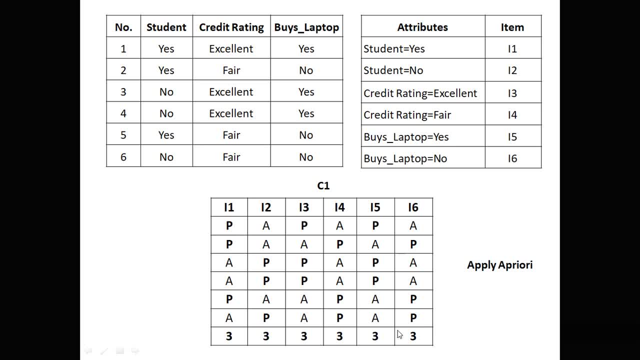 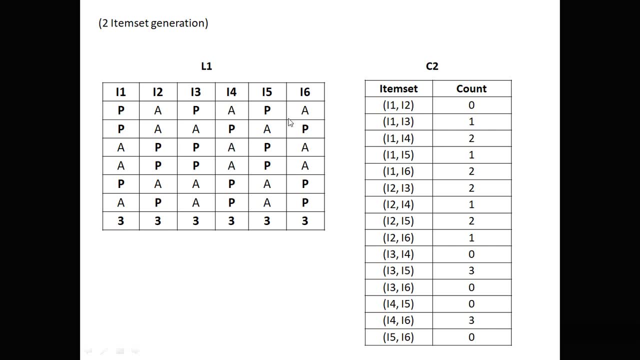 of a and b and the five at the bottom. we can write down the count as our minimum support count is one. so all get qualified into the l1. so this is our l1. now from l1 we generate the c2, that is two item set combination, and we are getting the combination from i1, i2 to i5, i6. in generation of c2 we exclude 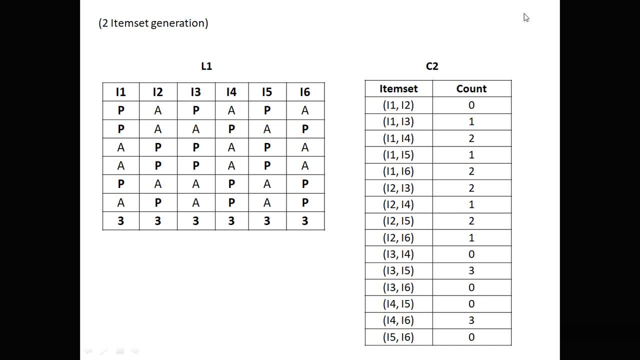 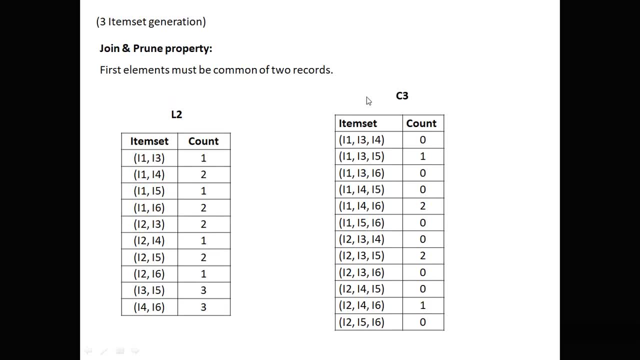 by the minimum support count. so here count is one. so we exclude all the items when there is minimal support value or count is zero. now from l2 we generate the c3, c3. this is the l2, this is c3. when we generate the three item set combination, we have to apply join and prune. property of a priori. i have 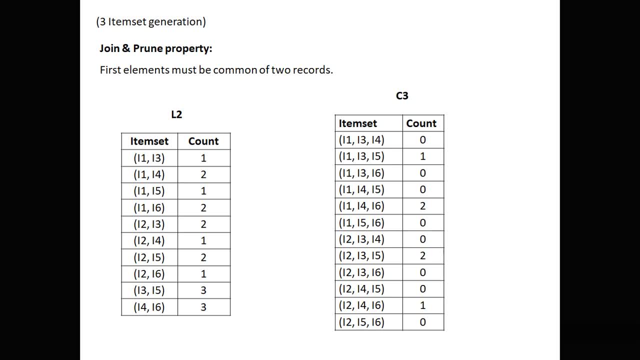 already published the videos on a priori. you can refer that videos for more information about join and prune property of a priori. for three item set generation. one at first item must be common so we can generate the rule from here. that is i1- i3, i1- i4, because first item is common but we can't generate the rule from i1- i3. 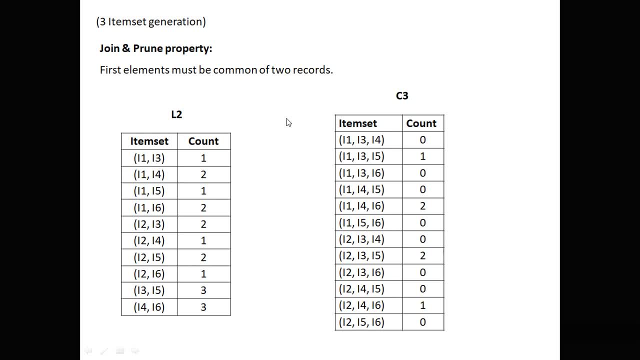 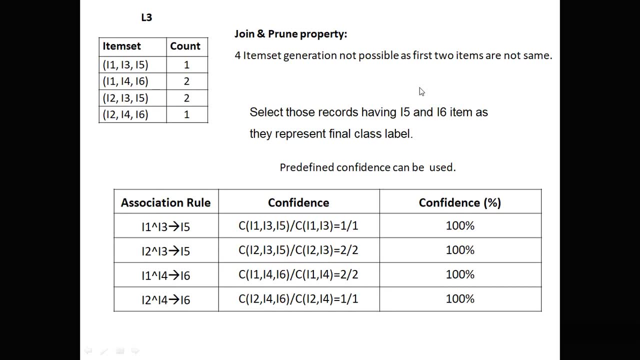 and i2, i3, because first item is not common. so in this way we require to take the combination using join function and write down the c3 set. now from c3 we generate the l3, so in l3 the qualified records which satisfy the minimum support count. now again we 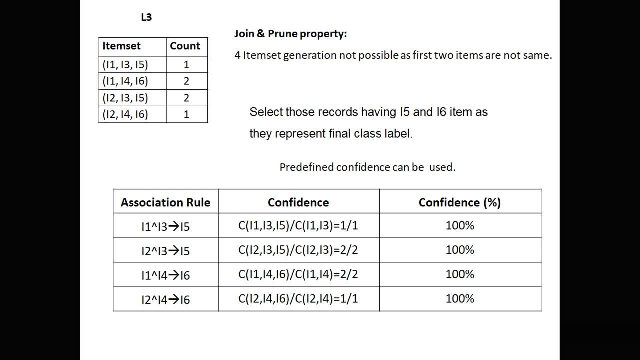 to generate the c4. but c4 is not possible because to generate the c4 we require that two items should be common: i1, i3- there is only one item is common, but no two items are common, so c4 can't generate and therefore there is no question of l4 now. l3 is our final large set. now here we can easily. 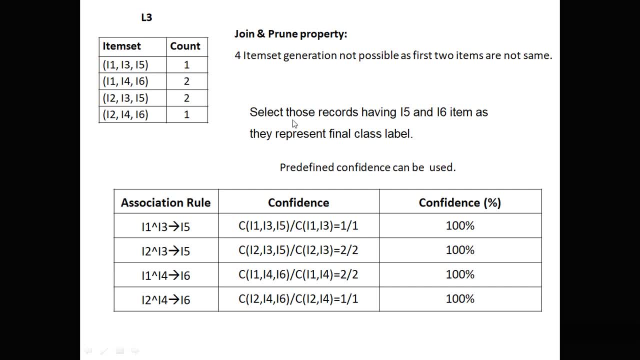 find out that i5 and i6- they are nothing but our final class level, because they belong, whether the laptop is purchased or not. that is why we require to apply to generate the c4. we need to generate the c4, to generate the c4, to generate the c4. 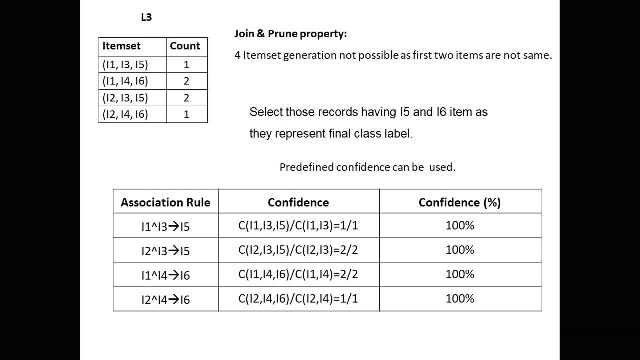 purchase or not, that is, by its laptop. therefore, these are the i6, and i6 are the final class level. now predefined confidence can be used. now the rules get satisfied, all or four. i have not written the very final rules. i have written only at the course level. but by applying or prior, you can. 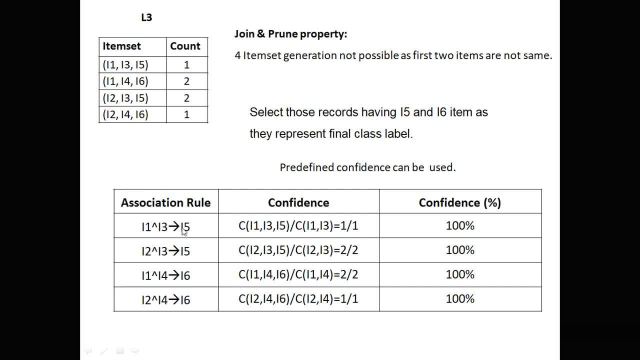 write down all the rules now here. the first rule is i1, i3, i5, i5 and i6 should be on the right hand side because they are nothing but our class level. i1- i3 implies i5, so count of i1- i3- i5 divided by i1.